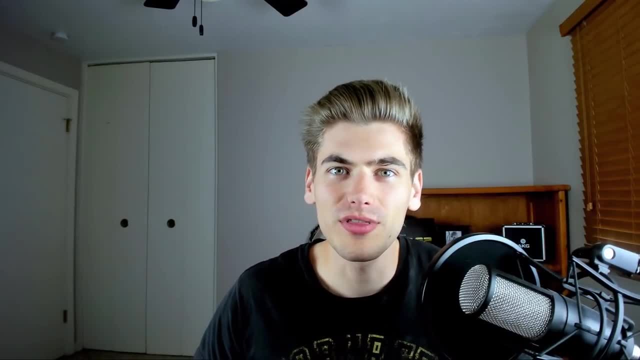 Hello everyone, In today's video, I'm going to be going over the facade pattern, which is one of my favorite design patterns available, because it really makes your code so much cleaner to write and also, most importantly, it makes it really easy to. 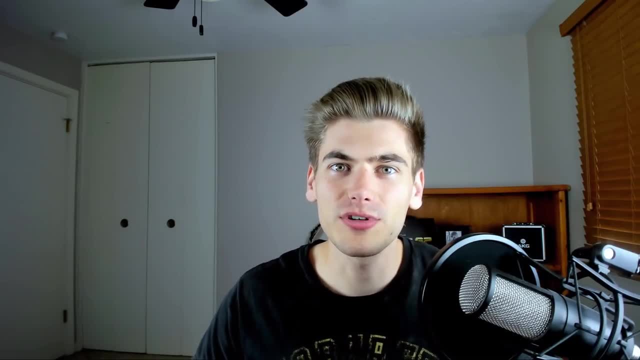 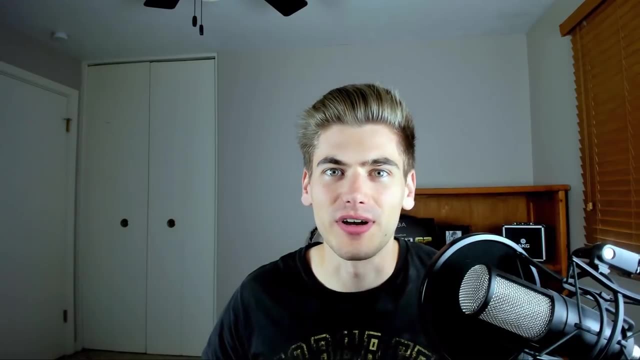 refactor your code in the future. So, without any further ado, let's get started now. Welcome back to Web Data Simplified. My name's Kyle and my job is to simplify the web for you so that you can start building your dream projects sooner. So if that sounds interesting, 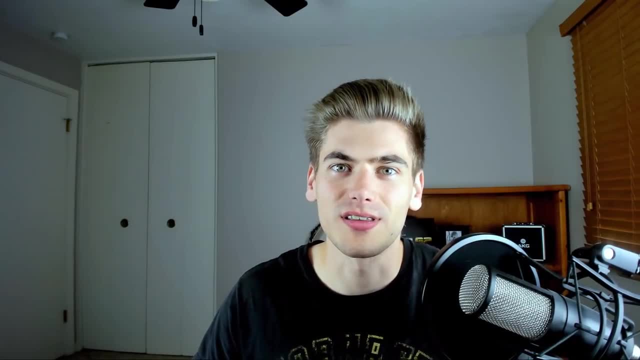 to you. make sure you subscribe to my channel for more videos just like this one. Now, before we jump into the code of the facade pattern, I first want to talk a little bit about what it is and why it's so important to use. 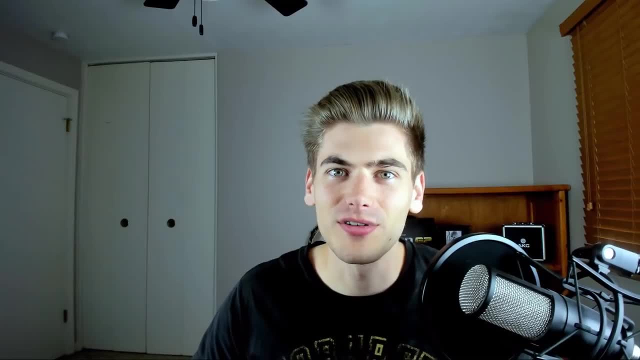 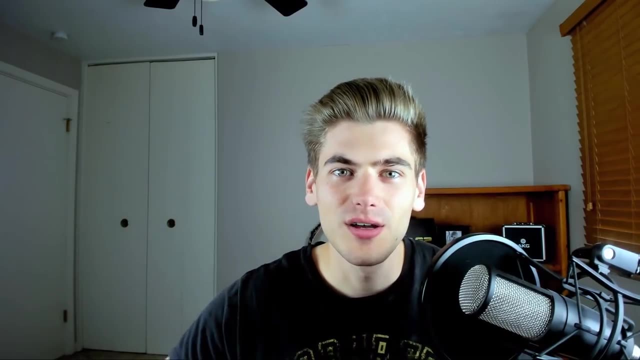 And essentially the entire idea behind the facade pattern is to make it easy for your code to change in the future. So the idea of this is that you create a facade between your complex code and your actual business logic code that you're writing. So a really good example. 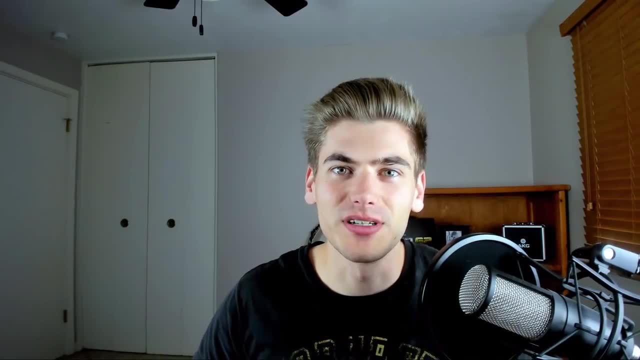 which is the code that we're going to be using, is the Fetch API built into the browser. It allows you to query APIs and get certain data from APIs, but it's kind of cumbersome to use and most likely you're going to trade it out later for something like Axios. 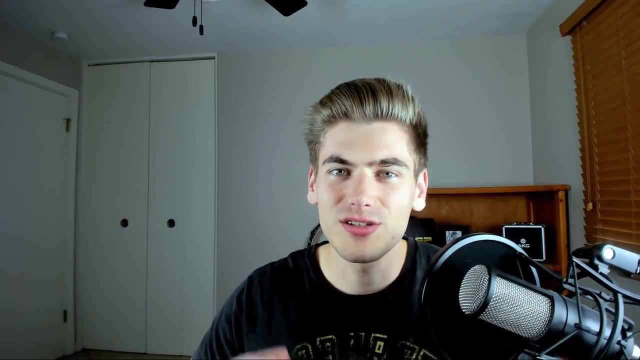 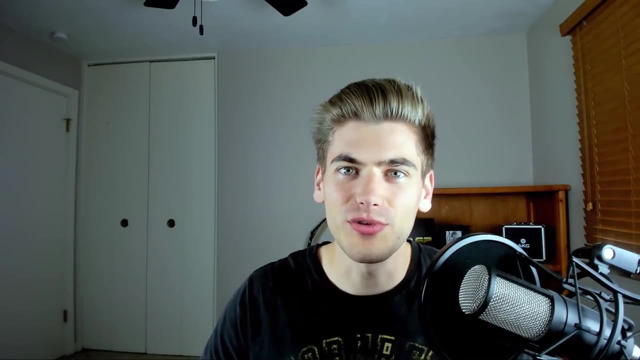 And the idea of the facade pattern is that not only does it make it so much easier to use these complex things such as Fetch, but it also makes it really really easy to replace in the future, which is, in my opinion, the reason it is so, so useful. 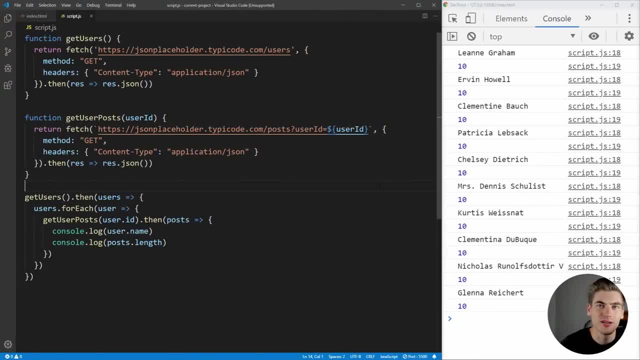 So let's jump into a code example. On the left side of my screen we have two functions, one for getting users and one for getting the user's post, And they're both very similar. They both call this Fetch API from the JSON placeholder API and they're getting users in. 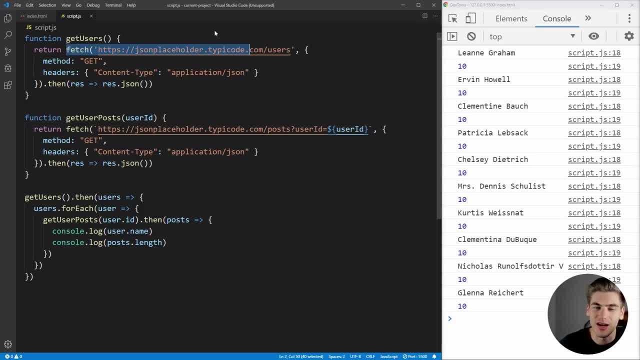 the first one and post in the second one, But all of the contents of this Fetch method are the same. We have the same method. We have these headers that we have to pass along to tell Fetch that we're actually getting the code, And then we have the code that we have to pass along to tell Fetch. 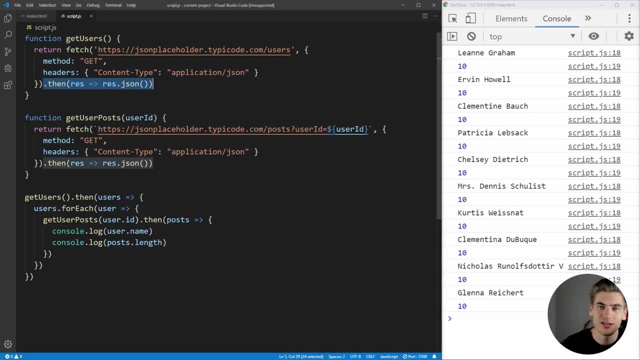 that we're actually getting the code. And then we have the code that we have to pass along to tell Fetch that we're actually getting JSON data, And then we're also converting that response to JSON so we can actually use it inside of our application. And this is a lot of code that's not really directly. 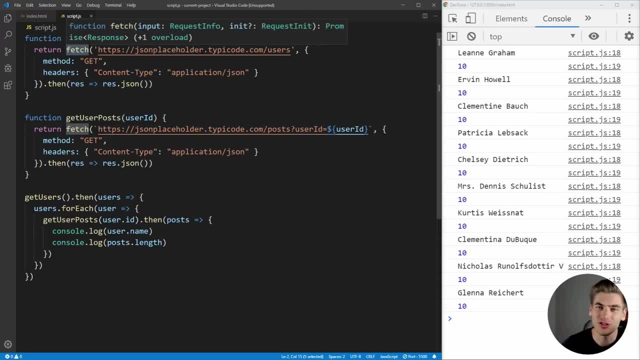 tied to getting a user. It's all kind of information that Fetch needs and the rest of your code really doesn't care about. So what we're going to do is implement the facade pattern and essentially create a facade between the implementation of Fetch and the actual API. we're 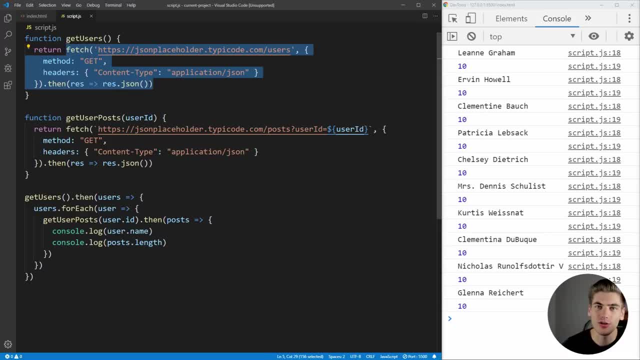 going to use inside of get users. So, essentially, we're going to create a function which does all of this information And all we have to do is pass it. the information that changes, such as, in our case, this URL is the thing that's different between this function and this function, And also 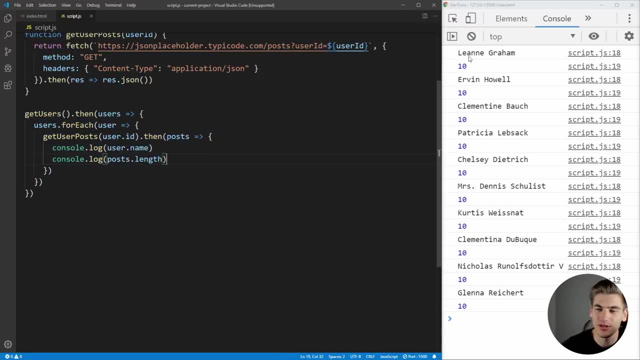 down here. all we're doing is looping through all of our users, getting their posts and then printing out their name and number of posts on the side, just so we can make sure that all the changes we make still work. So we should get the same output later on. So let's create that. 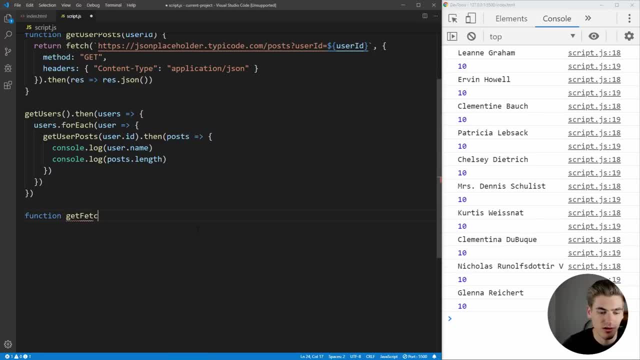 function. Now we're just going to call it get fetch, And this is going to take a URL. As you can see, here we have our URL And we're also going to take parameters, Because this is actually passing parameters to our URL. So let's take the URL and the params. 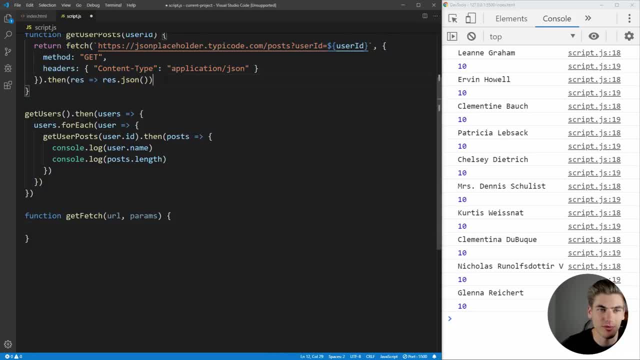 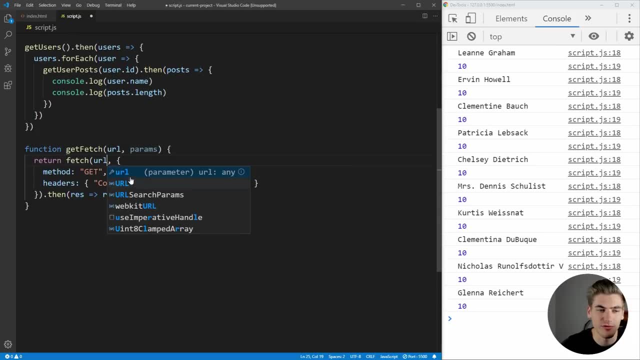 And what we want to do is a very similar thing to up here. So let's just copy all of this code for fetch, paste it into our git fetch And you can replace this entire section with our URL, because we want to fetch for a particular URL. we want to make sure that we're using git. 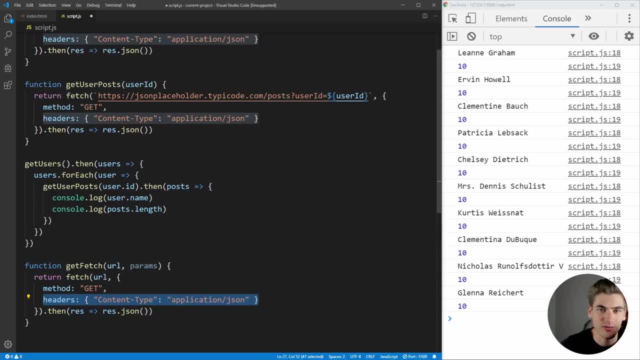 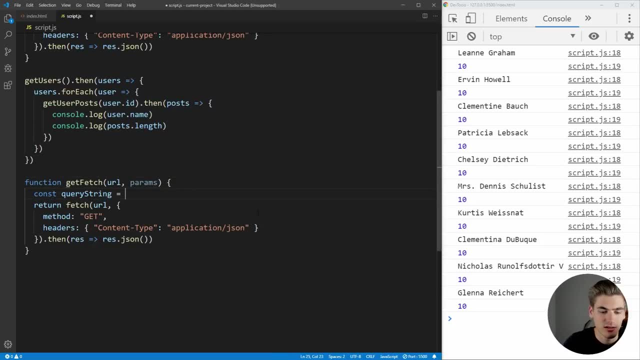 And we're sending that content. type of application: JSON. The last thing we had to do is just append our params onto the end of the query string So we can just get our query string here is going to be equal to object dot entries for params, Because what we're going to do is params. 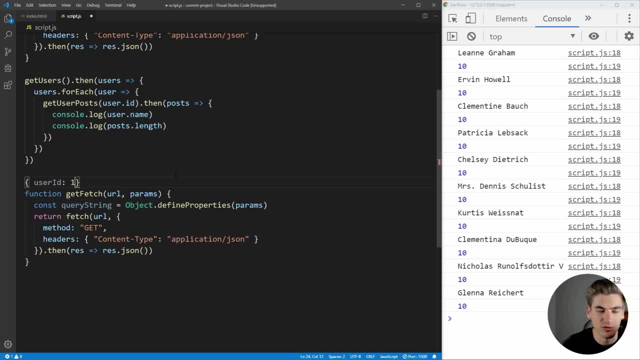 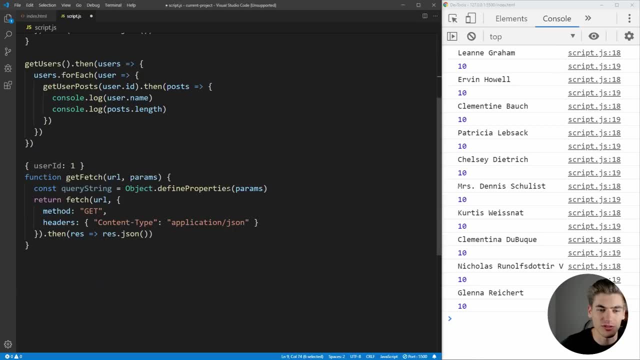 is going to look something like this. it's going to say user ID is equal to one, for example. So the key is going to be the actual parameter case here, user ID, And this value is going to be the value after the equal sign. So by saying here, object, dot entries, what we're doing is we're 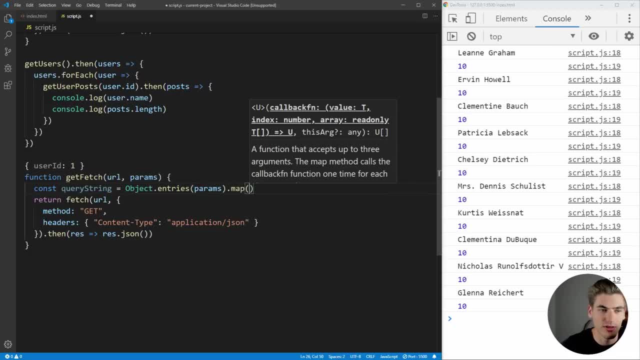 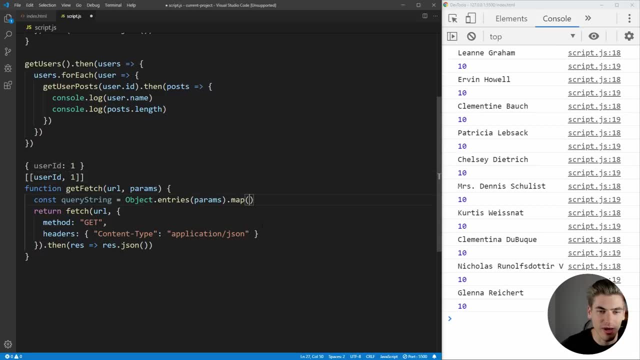 getting an array for each one of these. So we're going to have here: this is going to be converted to an array, And inside of that array we're going to have user ID and one just like this, So we can just map over that. So we're going to have a param And for 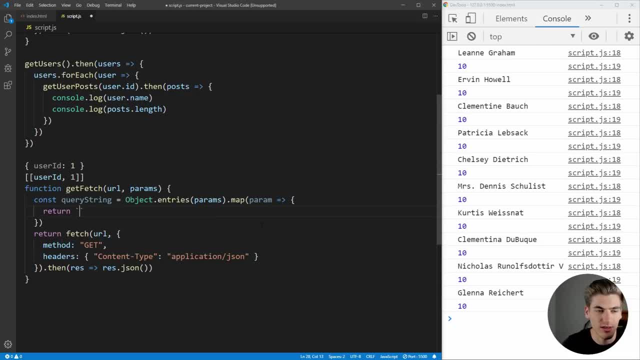 each one of our params. all we want to do is return a string And that string is just going to have, at the very beginning, it's going to have our param of zero, which in our case is user ID, And then we want to say equal, And then we want to get param here of one And that param one is going. 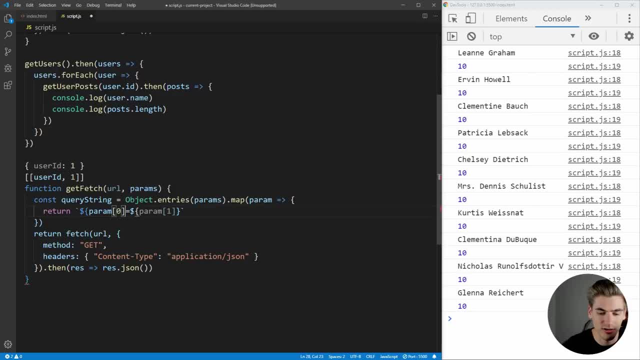 to be equal to our user ID. In this case it's just one. So now let's close that all off, And the last thing we want to do is just join this array together on the and symbol. So essentially we're concatenating them all to create a correct query string, And this code right here doesn't. 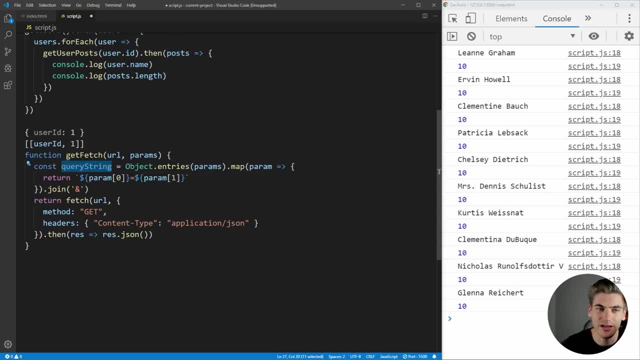 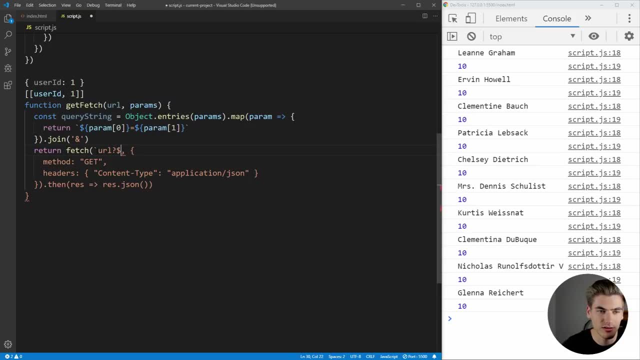 really matter too much. It's just implementation of the fetch function, which we're trying to hide from the rest of our program. Now we can just append this to the end of our query or URL, just by adding it in like this: paste that down and close it off, And now we can replace our get. 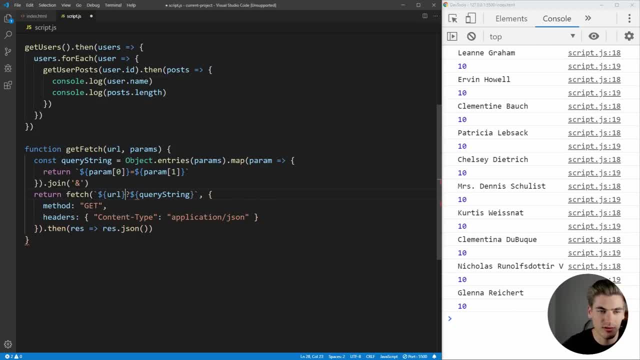 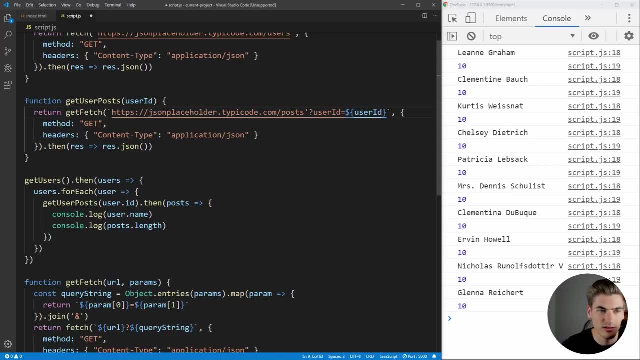 fetches Also. make sure that this is properly. Now let's replace our fetches up here with get fetch And we can just remove this, Just like whoops. that and all the code inside of here we no longer need. we just need to pass. 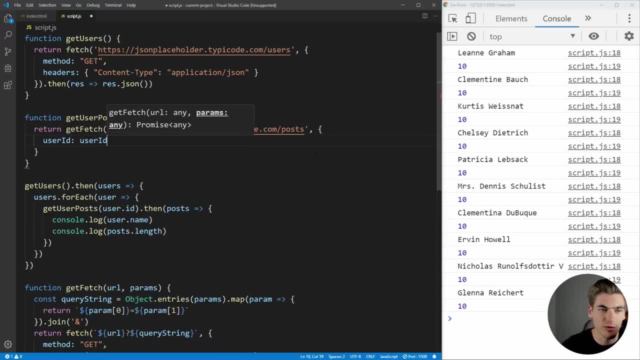 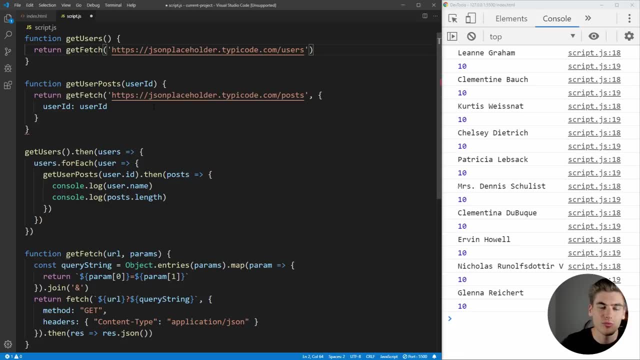 it our user ID, which is equal to the user ID parameter we're passing to this function. we can do the same thing up here, But we don't need any of this code down here. we can just remove all that So immediately. you see that with this facade pattern, 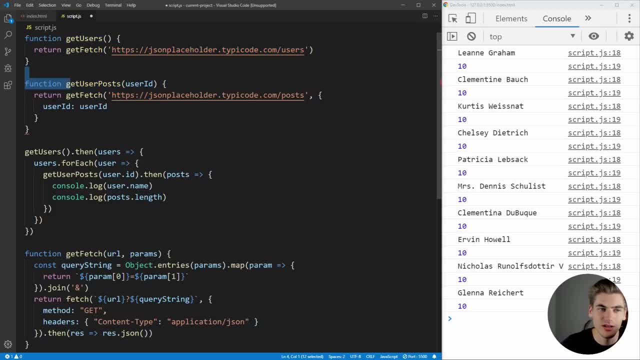 we've cleaned up our fetch functions for get users and get user post. Really simple just says get fetch, we pass the URL and we pass a parameters. That is just logical code that makes sense to read. We've made our API cleaner By creating this facade. This contains: 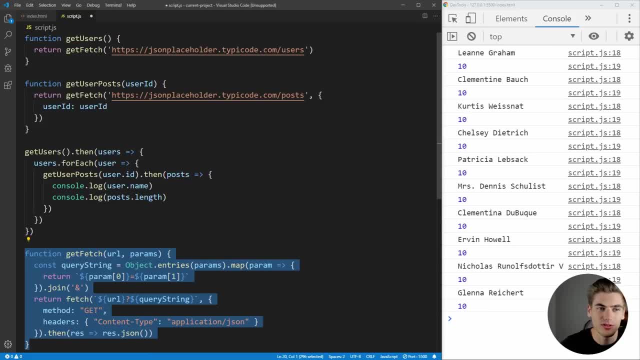 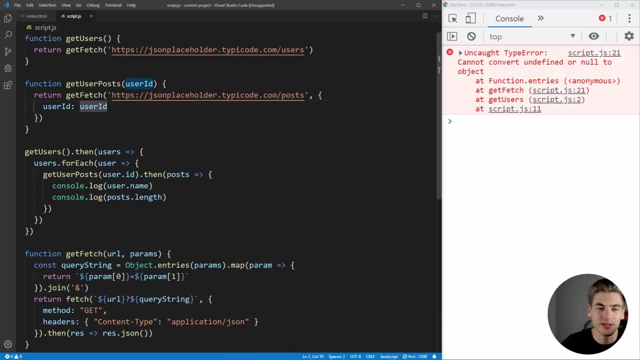 all of our ugly code that connects to fetch And it outputs just these clean code that we can use inside of our application. And if we say that, you can see we're getting an error over here. And that is because, by default, params is going to be null. So we want to just make sure we set. 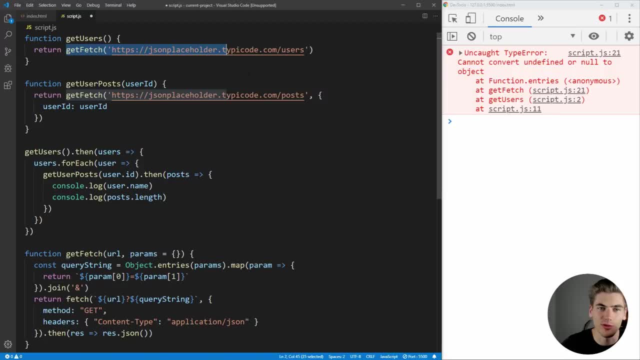 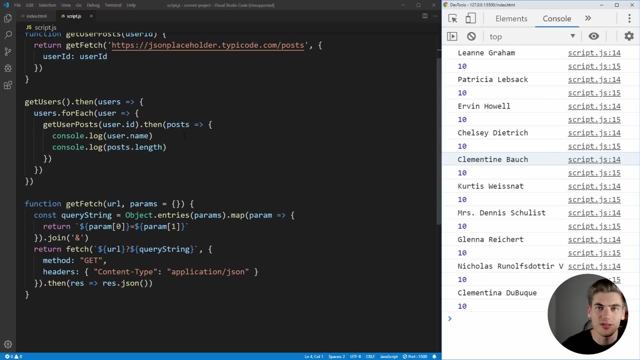 that to an object by default. if we don't pass one In this example, we don't pass params. Now if we say that, you can see, we're getting the people's names and the number of posts that they written. So already we've seen one of the big advantages of the facade pattern, and that it cleans up all. 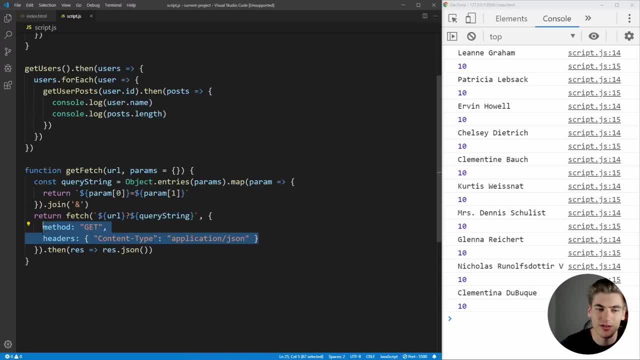 of our code. we no longer have to copy paste all this headers and methods stuff all over the place. It's all hidden away In one part of our code. we can even put this in some other module somewhere and we can import it anytime we need it, And it just cleans up our code to look much nicer and 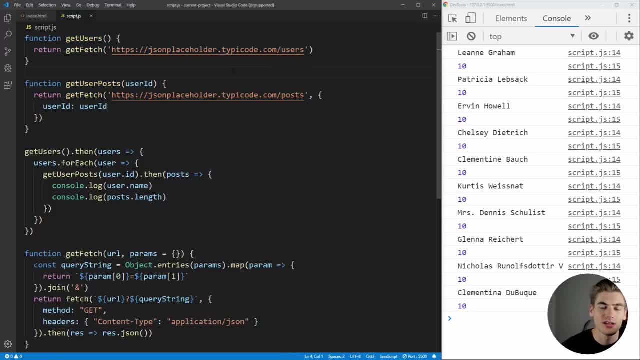 easier to write, But one of the really big advantages is when you want to actually change the implementation. If we want to change the implementation, we can just click on the command line, And if we wanted to change to use Axios instead of fetch. now that we have this, 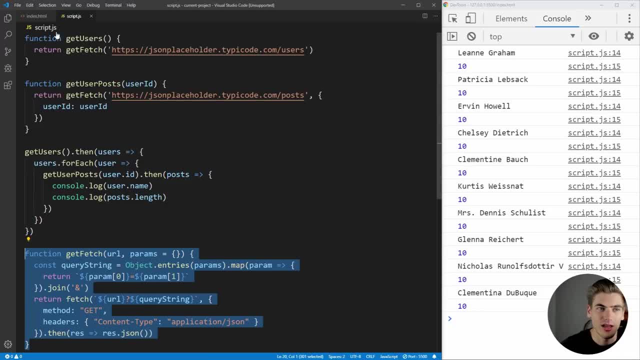 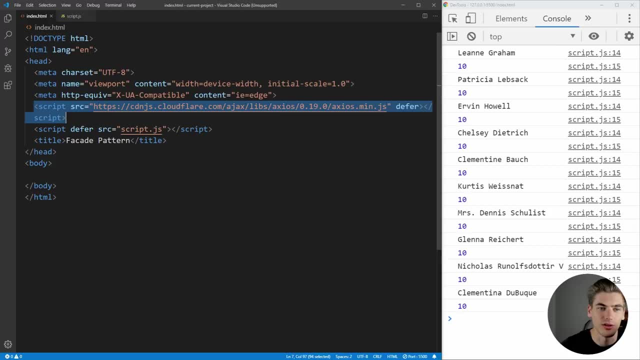 facade setup. it's actually really easy to do And I've already imported Axios into here. I have the script tag from the CDN. you can include this into your own application if you're following along. But anyway, all we need to do is we'll just copy this get fetch for now, So we can see both of them. 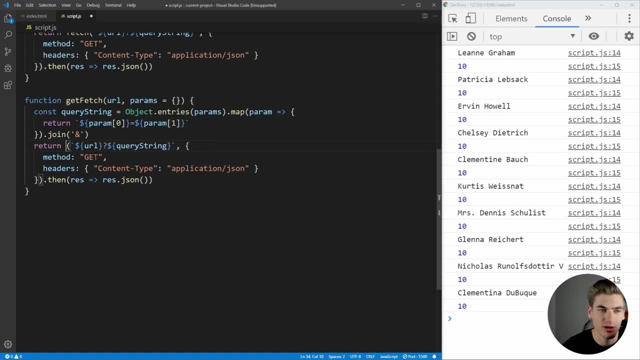 side by side And we can just replace our fetch here with a call to Axios, And the way Axios works is you actually just pass it an object, So we have our URL, which is our URL, And then we can. we're going to have our method, which is get, And we're also not needing to pass any headers, all. 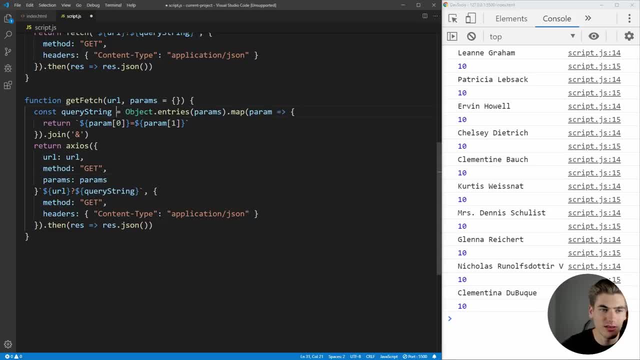 we can just pass in the params like this And we don't even need this query string at all. So now all we need to do is just do this final dot then. But in our case for Axios, we just return rez dot data And that's going to be the same as rez dot JSON for fetch. 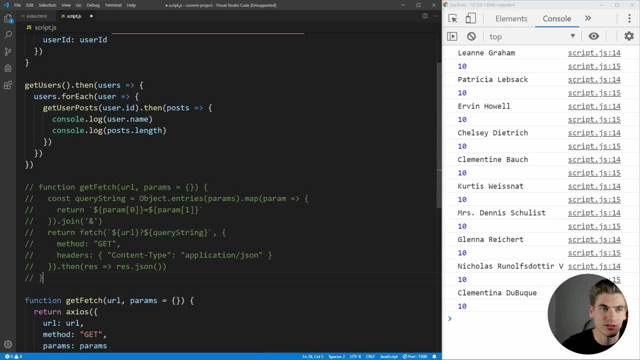 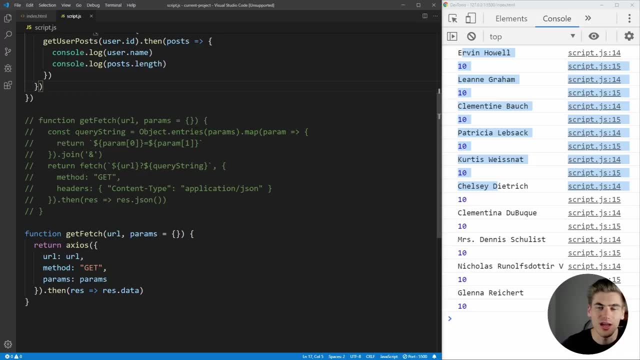 Now it's comment out this code here and actually make sure that this works. So if we save this, you can see on the side we're still getting all of our results. But now we're actually using Axios instead of fetch, And it was so easy to change over. we only had to change it in one place. 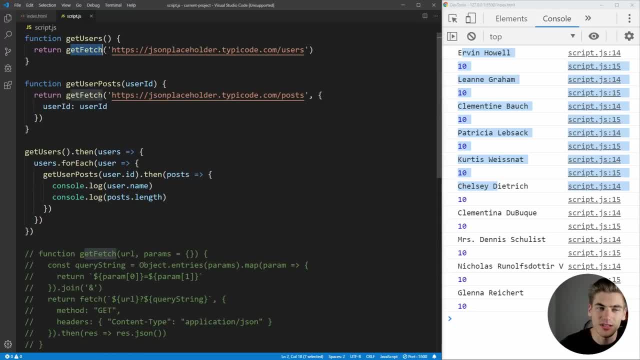 While if we had our old code, like at the beginning, we'd have to go to every single place in our code where we used fetch and replace it with Axios, And that's very, very error prone. you're bound to make mistakes doing that, But with this facade pattern.